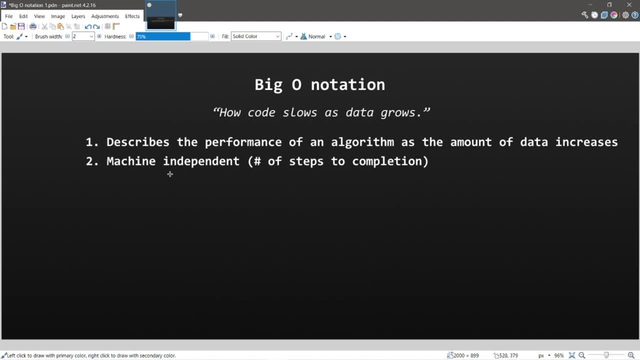 because some machines are going to run certain algorithms faster than others. And three, we tend to ignore smaller operations. If we had some task that took n plus one, we would just reduce it to just n, because that plus one really isn't going to make a difference. 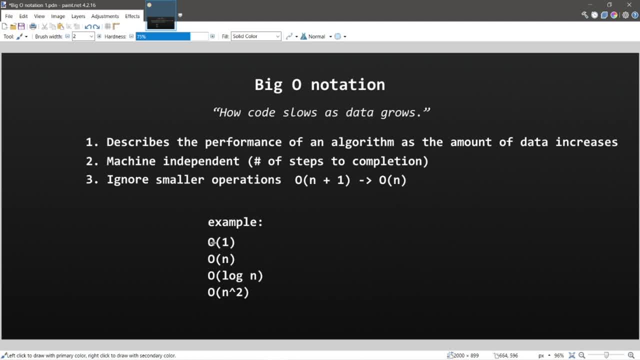 So here's a few examples of Big O Notation: We have O of 1, O of n, O of log n and O of n squared. And n is really just the amount of data that we're passing in. It's a variable like x. What we're focusing on is the performance of an algorithm as the amount of data increases. 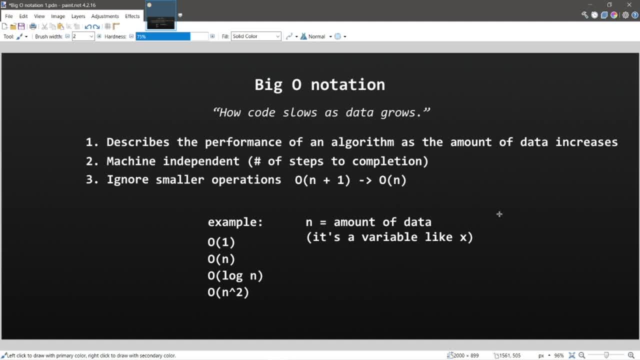 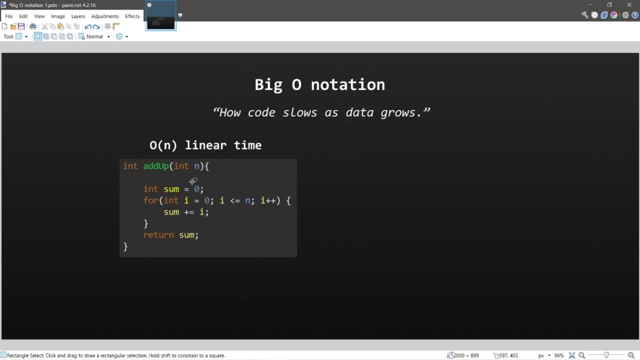 And n is a representation of the amount of data that we're passing in. Here's a more concrete example. I have a function named addUp. We will add up to a certain number, depending on what we pass in as an argument. The for loop within here will iterate once up to whatever number that n is. add i to sum, then return it. 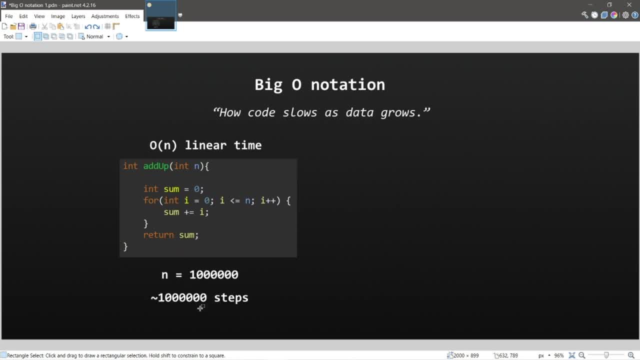 What if n was a large number like a million? Well, it's going to take just above a million steps to complete this function. This function is said to have a runtime complexity of O of n linear time. As the amount of data increases, it's going to increase the amount of steps linearly or proportionally. 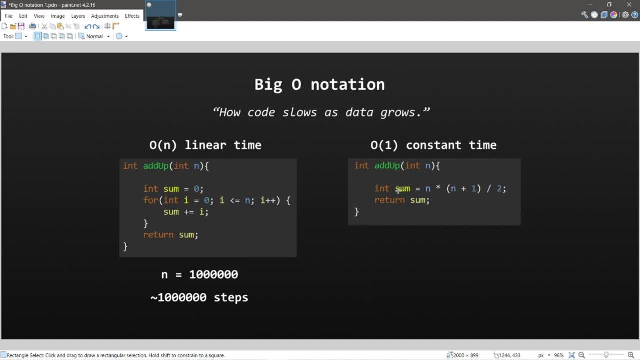 Now, another way in which we could write the same function is to take: sum equals n times n, plus one divided by two, We will get the exact same sum. So if n was, let's say, a million, this is still only going to take a couple steps. 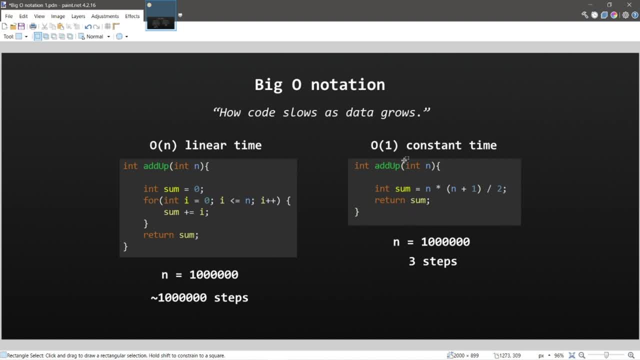 Three steps, not a million steps. So this function is going to have a runtime complexity of O of 1.. The input size doesn't matter. The amount of data that we have really doesn't matter. It's going to be completed in the same amount of steps. 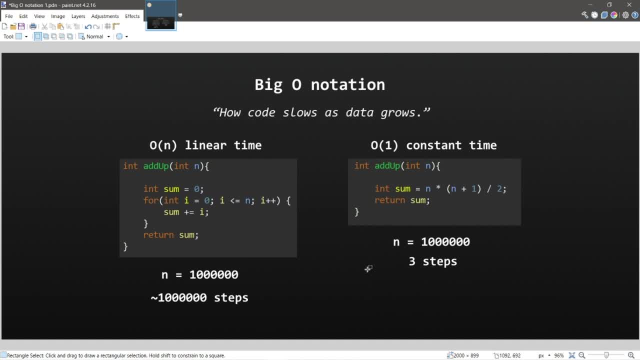 So this function is way better than this previous one. Three steps is better than a million steps, And the reason that this isn't O of 3, because this takes three steps- is that we really don't care about smaller operations. In the grand scheme of things, they really won't make much of a difference. 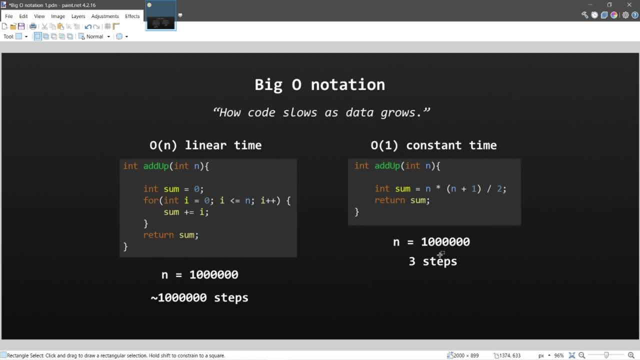 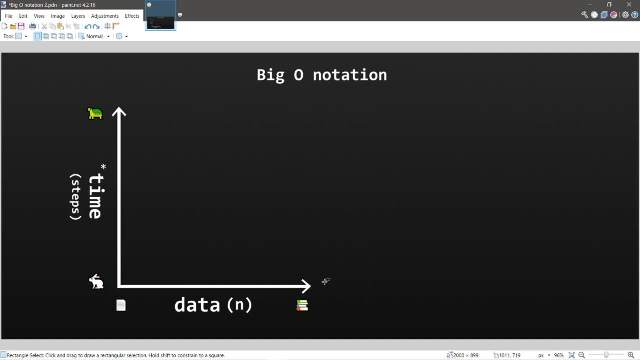 So we would just shorten this and say that this is O of 1 constant time. The input size doesn't matter. Here's a graph that I made to represent the different runtime complexities. We have data on the x-axis represented by n, So data will increase as we go more to the right. 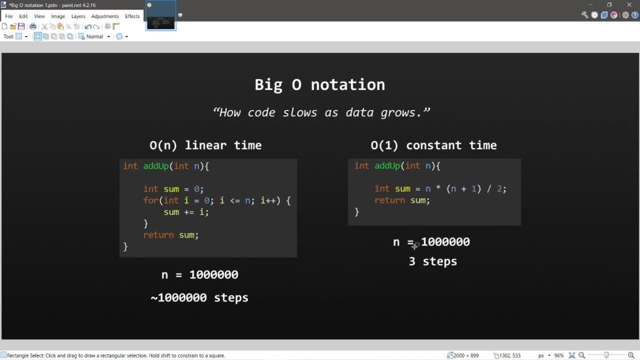 divided by the number of steps we're passing in. So we're going to have a by 2, we will get the exact same sum. so if n was, let's say, a million, this is still only going to take a couple steps, three steps, not a million steps. so this: 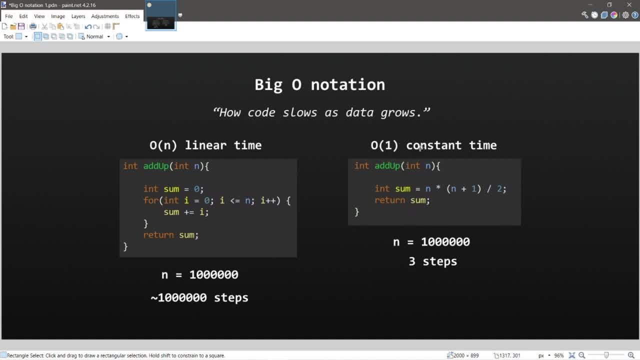 function is going to have a runtime complexity of O. the input size doesn't matter. the amount of data that we have really doesn't matter. it's going to be completed in the same amount of steps. so this function is way better than this previous one. three steps is better than a million steps, and the 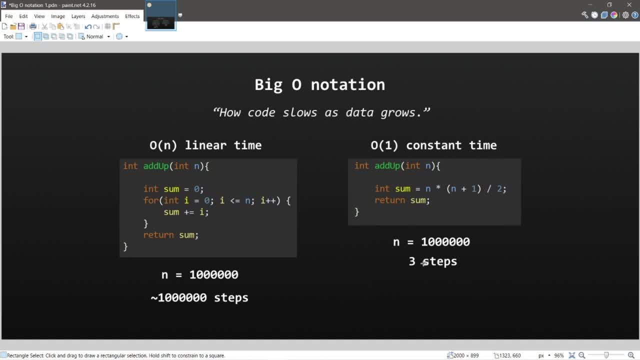 reason that this isn't O, because this takes three steps, is that we really don't care about smaller operations. in the grand scheme of things, they really won't make much of a difference. so we would just shorten this and say that this is O constant time. the input size doesn't matter. 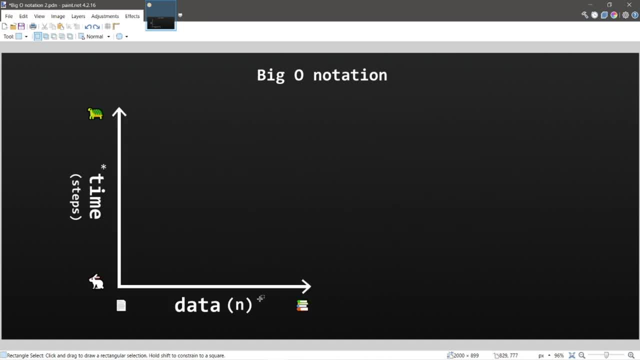 here's a graph that I made to represent the different runtime complexities. we have data on the x-axis, represented by n, so data will increase as we go more to the right and we have time on the y-axis. I did add an asterisk next to time. 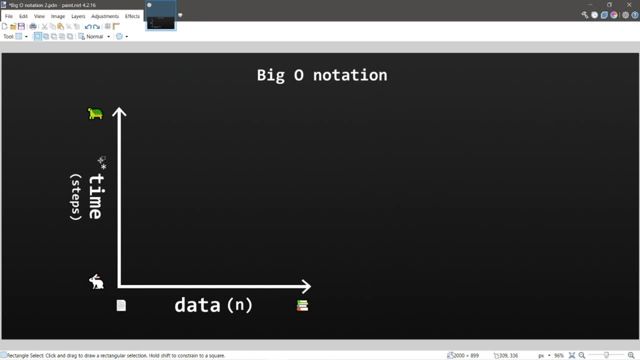 because that's what we're going to be doing next. so we're going to be doing some of these times depending on what machine you're using, so these can vary. another way to look at this is number of steps, so as we increase on the y-axis. 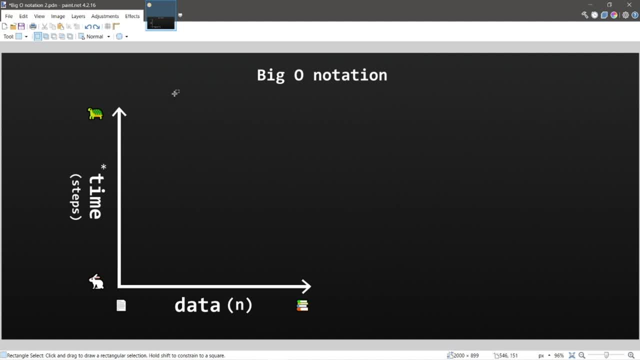 these algorithms are going to perform with increasingly more time. they're going to get slower. so let's begin with O, constant time. anything that has a runtime complexity of O will take the same amount of time, regardless of the data size. a few examples would include the random. 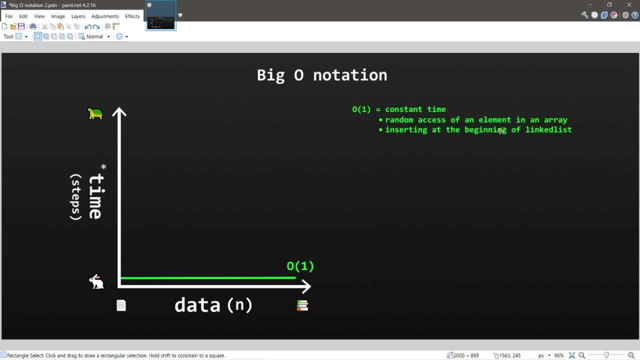 access of an element within an array and inserting at the beginning of the list. so O is extremely fast. next, we have O, also known as logarithmic time. one example is binary search. we haven't talked about this yet. we'll talk about a few of these algorithms in future videos, but anything 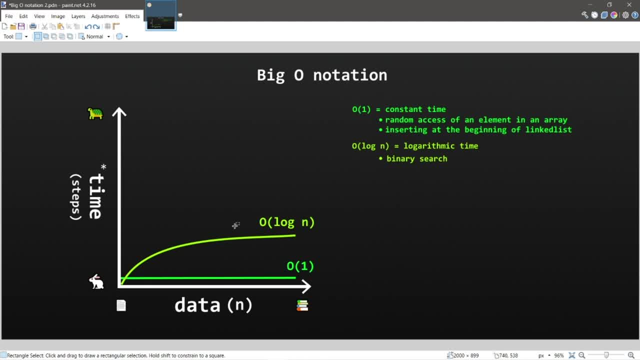 that has a runtime. complexity of O will actually take- I don't want to say less and less time, but increasingly less time- to complete. so as the data size increases, this algorithm is going to be more and more efficient compared to the early stages with a small data set. O is also known as linear time. 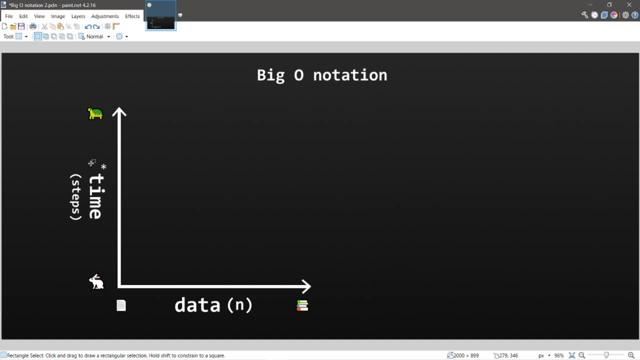 And we have time on the y-axis. I did add an asterisk next to time because some of these times can vary depending on what machine you're using. So if we go to the right, we have time on the y-axis, So these can vary. 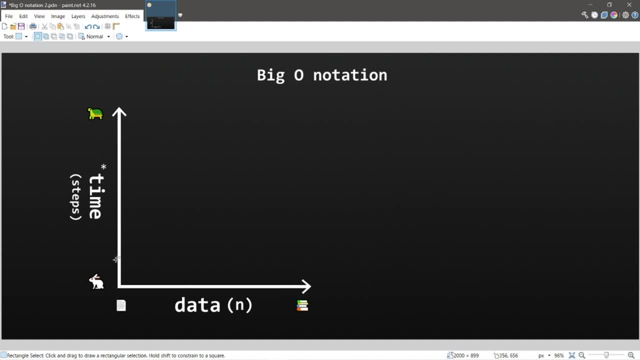 Another way to look at this is number of steps. So as we increase on the y-axis, these algorithms are going to perform. with increasingly more time, They're going to get slower. So let's begin with O of 1. constant time: Anything that has a runtime. complexity of O of 1. 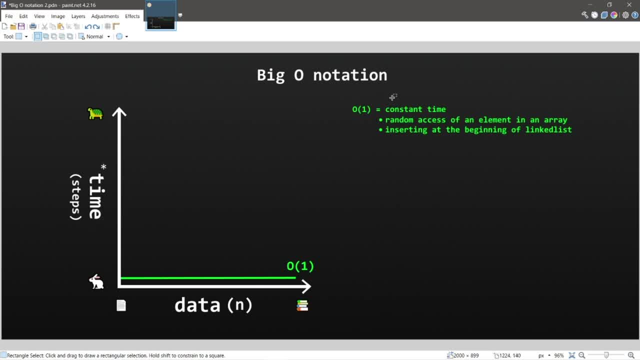 will take the same amount of time regardless of the data size. A few examples would include the random access of an element within an array and inserting at the beginning of a linked list. So O of 1 is extremely fast. Next we have O of log n, also known as logarithmic time. 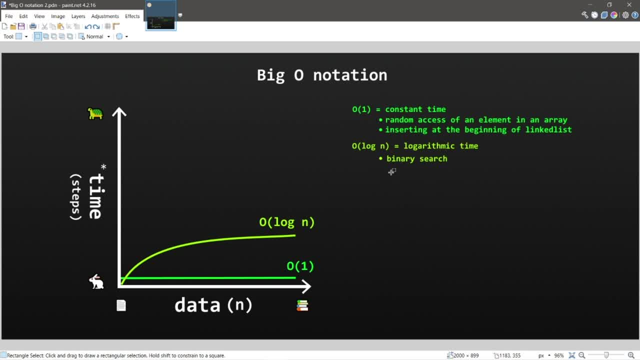 One example is binary search. We haven't talked about this yet. We'll talk about a few of these algorithms in future videos. But anything that has a runtime complexity of O, of log n will actually take, I don't want to say less and less time. 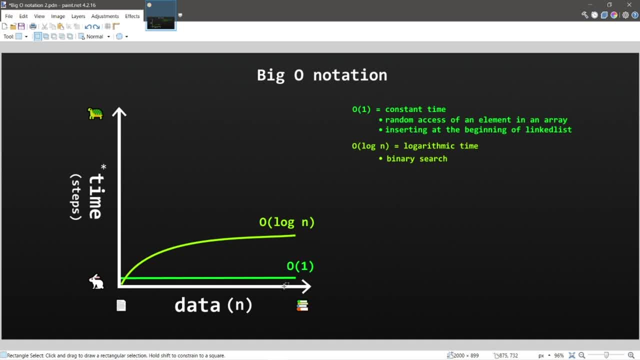 but increasingly less time to complete. So as the data size increases, this algorithm is going to be more and more efficient compared to the early stages with a small data set. O of n is also known as logarithmic time, So O of n is going to be more and more efficient. 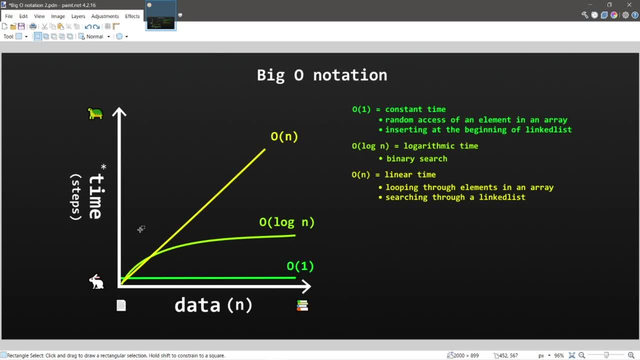 O of n is also known as linear time. As the amount of data increases, the time it takes to complete something will increase proportionally linearly. That would include looping through the elements in an array and searching through a linked list. Next we have O of n, log n, also known as quasi-linear time. 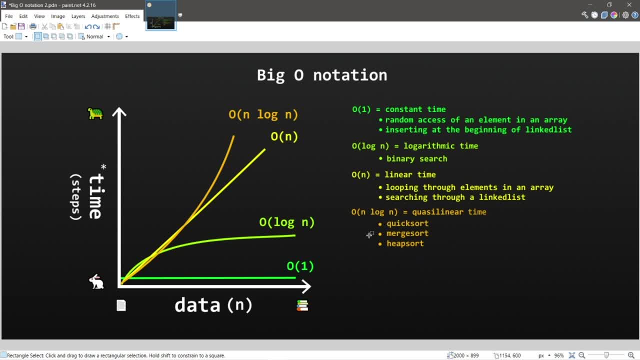 This would include a quick sort, merge sort and heap sort. We'll talk about these concepts in future videos. So for the most part this is very similar to linear time. unless we're working with a large data set, Then anything using O of n log n is going to start to slow down. 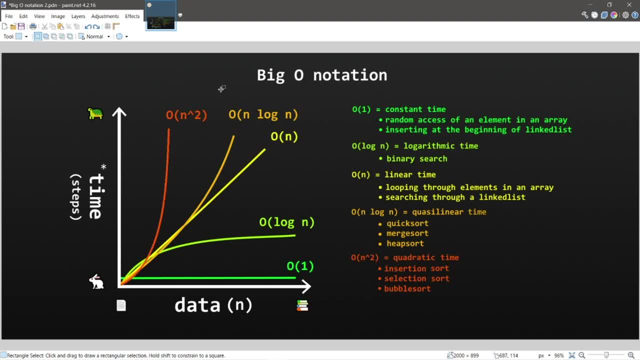 when we work with larger data sets, hence this curve here. Then we have O of n squared, also known as quadratic time. A few examples would include insertion sort, selection sort and bubble sort. As the amount of data increases, it's going to take increasingly more and more time. 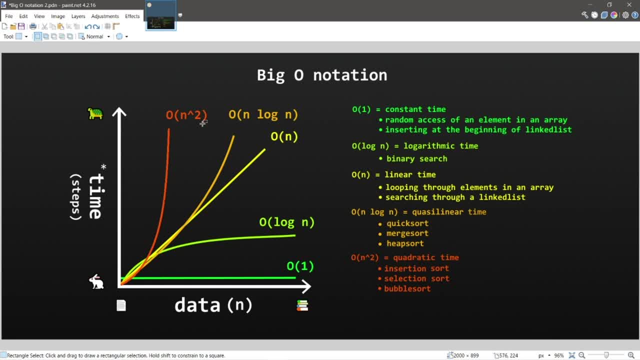 to complete anything that has a runtime. complexity of O of n squared. So just to compare linear time and quadratic time: with linear time it's going to take more and more time to complete anything that has a runtime. complexity of O of n squared. 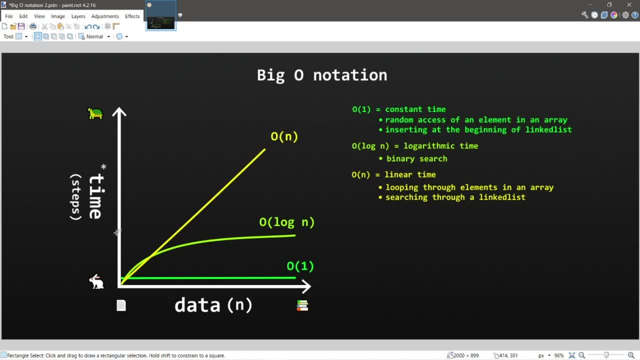 as the amount of data increases, the time it takes to complete something will increase proportionally. linearly, that would include looping through the elements in an array and searching through a linked list. next we have O, also known as quasi-linear time. this would include a quicksort, merge sort. 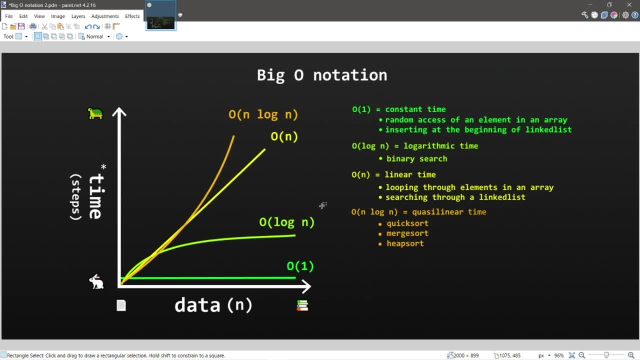 and heapsort. we'll talk about these concepts in future videos. so for the most part, O is only used for linear time. unless we're working with a large data set, then anything using O is going to start to slow down when we work. 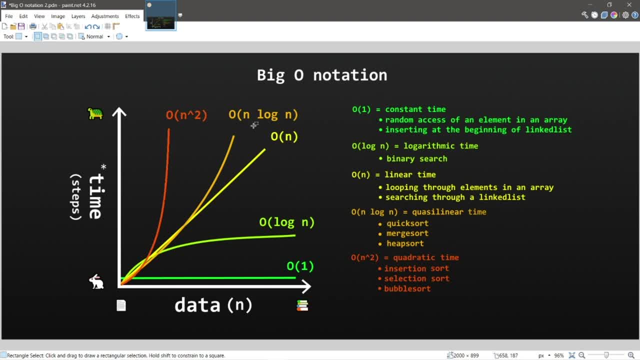 with larger data sets, hence this curve here. then we have O, also known as quadratic time. a few examples would include insertion, sort, selection sort and bubble sort. as the amount of data increases, it's going to take increasingly more and more time to complete anything that has a runtime. complexity of O. 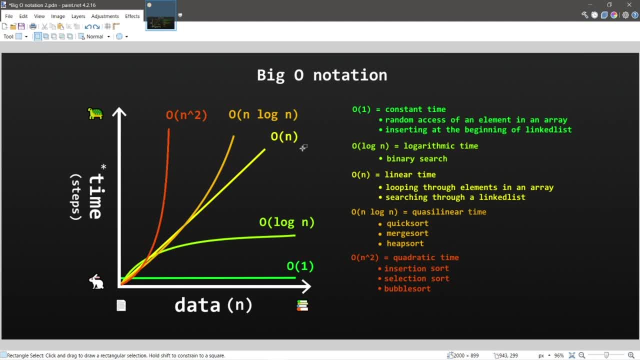 linear time and quadratic time. With linear time, if our data set was a thousand, if n equals a thousand, it's going to take a thousand steps. They're proportional, they're linear. but if we were using quadratic time, if n was a thousand, then a thousand squared would be a million. So if 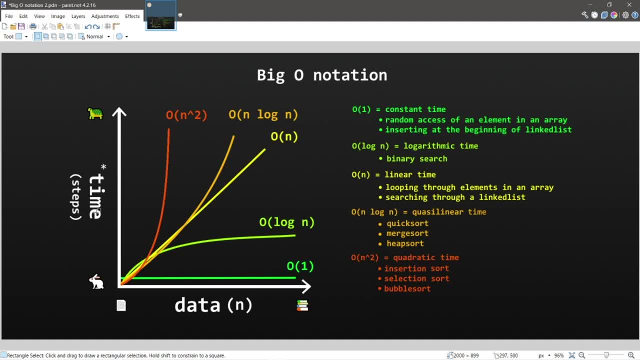 our data set was a thousand. if we're using quadratic time it's going to take a million steps then- way more than linear time. So quadratic time is extremely slow with large data sets, but in the case of a small data set it could actually be faster, as you can see by the graph here And 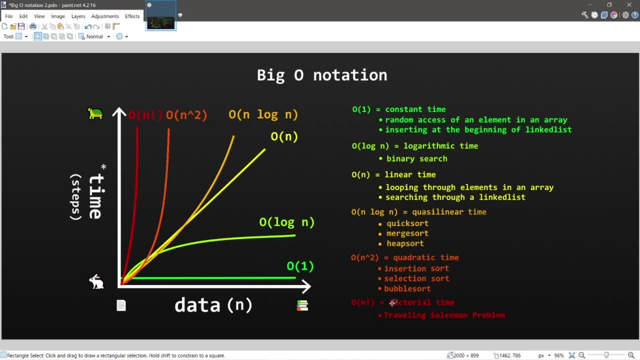 lastly, we have O of n- factorial, also known as factorial time, and one place where this is used is with the traveling salesman problem, which I might discuss in a future video. So this is extremely slow. So if I had to give a letter grade to each of these runtime complexities when working with 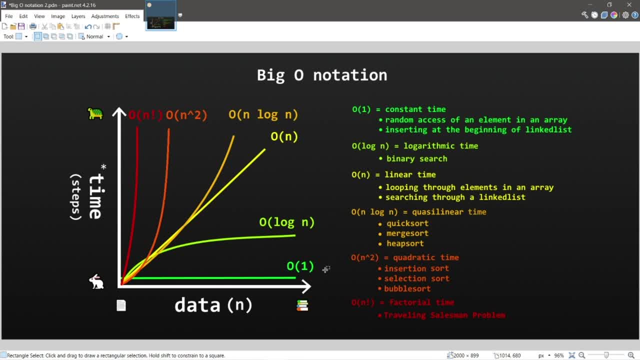 large data sets with constant time. this would be an a like an a, plus Logarithmic time would be a- b, it's pretty good. Linear time: it's c, it's okay. Quasilinear time is a- d, it's just barely passing. Quadratic time would be an f. 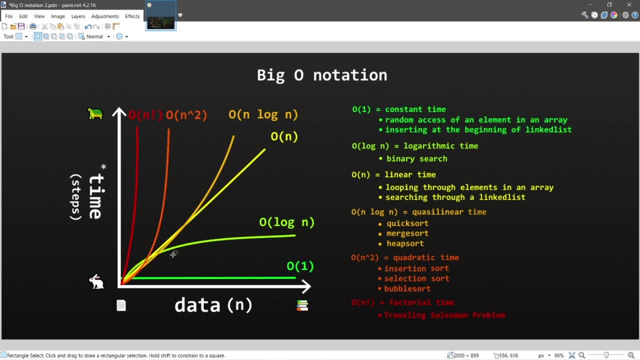 and factorial time. well, you get expelled from school, Although some of these runtime complexities are actually faster when working with a smaller data set. so keep that in mind. Well, that's the very basics of big O notation. It's notation used to describe the performance. 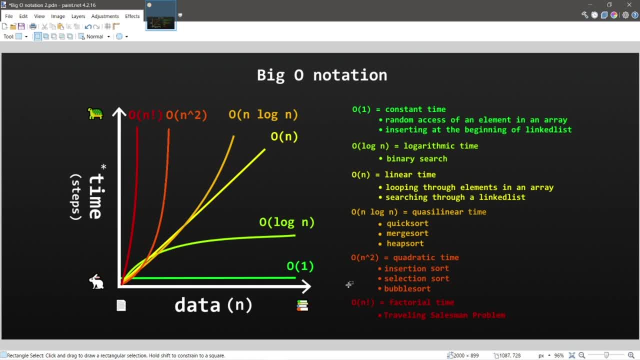 of an algorithm as the amount of data increases. So if you can give this video a thumbs up, drop a like and I'll see you in the next video. And well, that's big O notation in computer science. 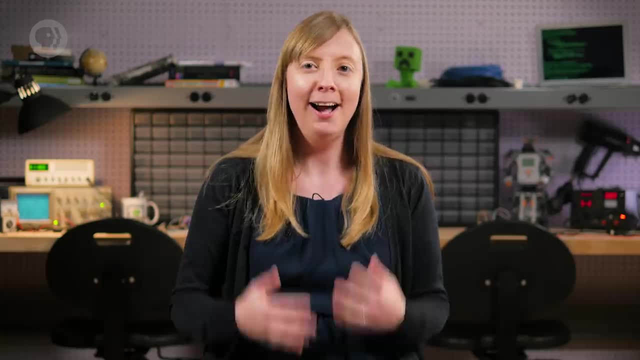 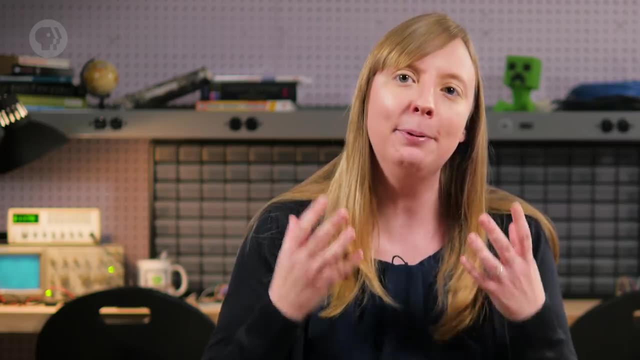 Hi, I'm Carrie-Anne and welcome to Crash Course Computer Science. Today we start our journey up the ladder of abstraction, where we leave behind the simplicity of being able to see every switch and gear but gain the ability to assemble increasingly complex systems. 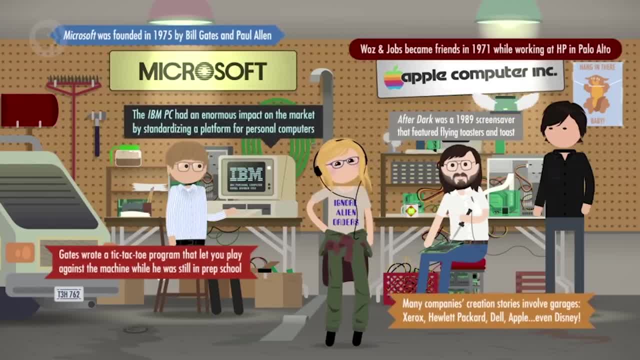 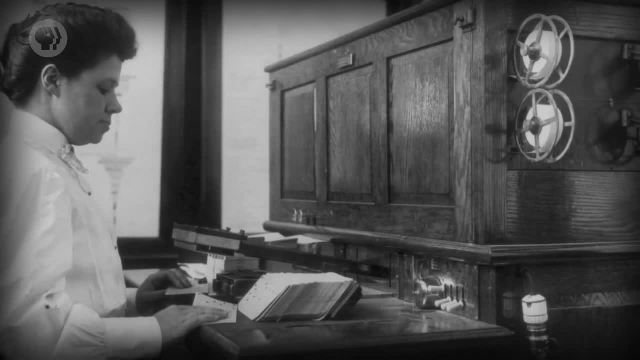 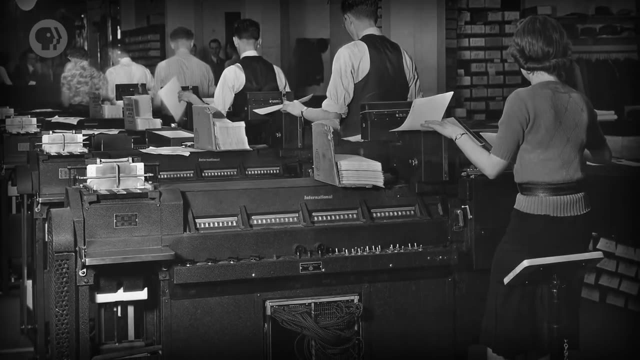 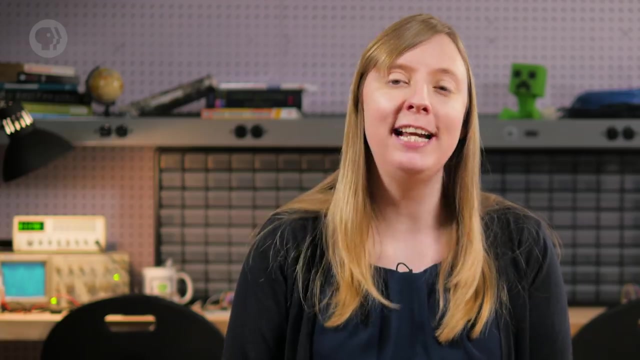 Last episode we talked about how computers evolved: from electromechanical devices that often had decimal representations of numbers, like those represented by teeth on a gear, to electronic computers with transistors that can turn the flow of electricity on or off. Unfortunately, even with just two states of electricity we can represent important information. 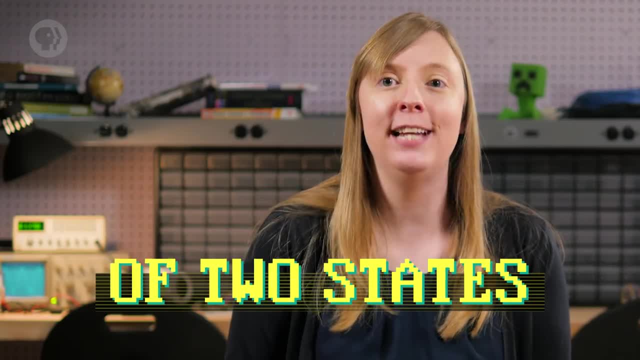 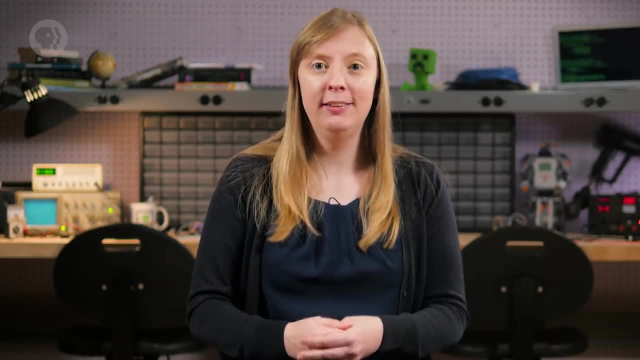 We call this representation binary, Which literally means of two states. in the same way, a bicycle has two wheels or a biped has two legs. You might think two states isn't a lot to work with, and you'd be right, but it's. 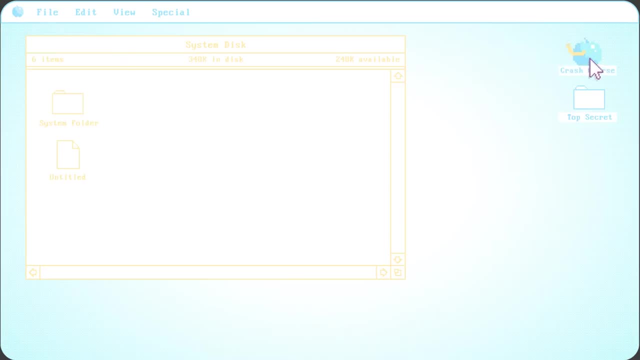 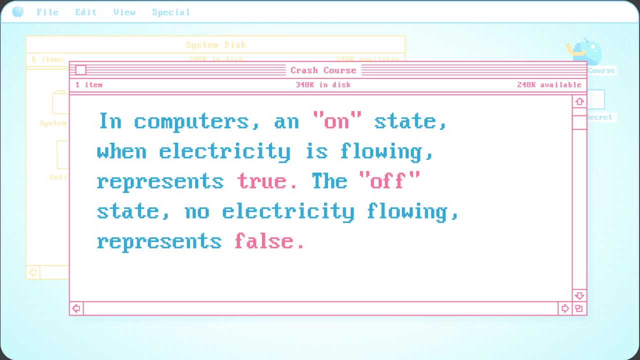 exactly what you need for representing the values true and false In computers. an on state when electricity is flowing represents true. The off state, no electricity flowing, represents false. We can also write binary as ones and zeros instead of trues and falses. 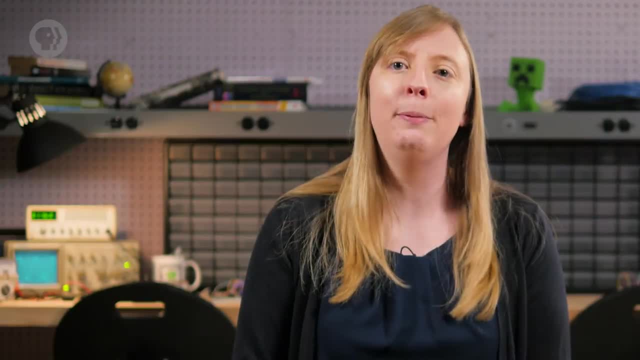 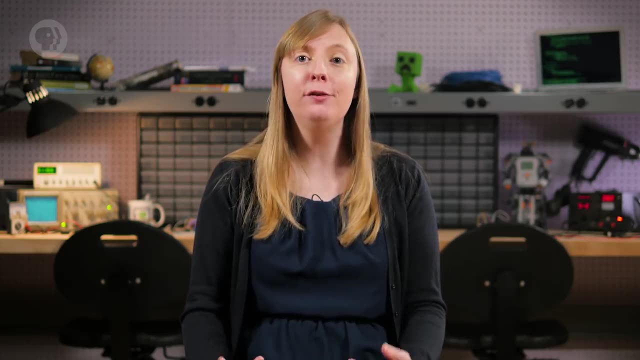 They are just different expressions of the same signal, But we'll talk about that in the next episode. Now it is actually possible. It's even possible to use transistors for more than just turning electrical current on and off and to allow for different levels of current.